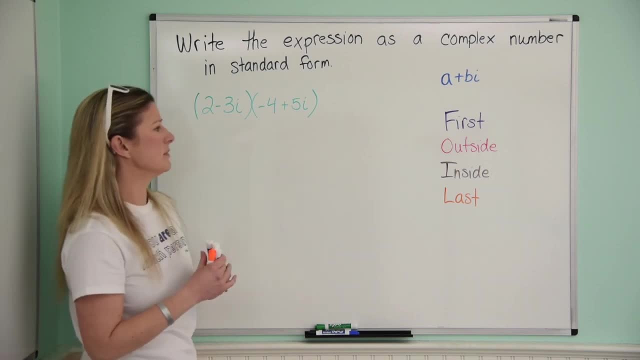 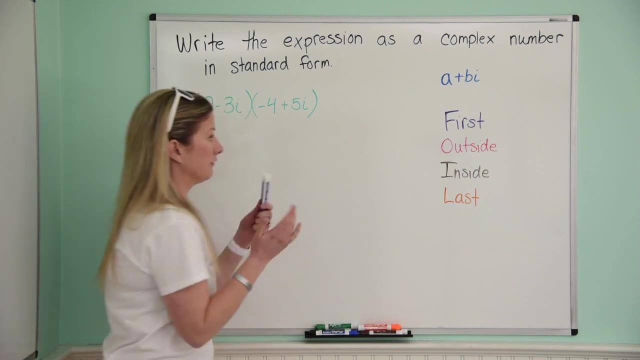 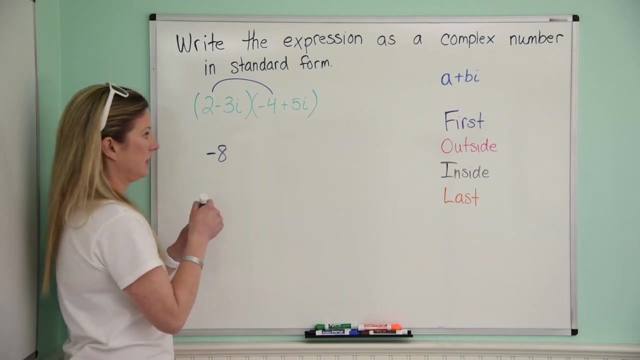 I've already got the green up there and the blue. Okay, awesome. So this is telling us which terms we're multiplying together. So first means we are multiplying the first two terms together. Okay, boom. So two times negative Four, That's going to be negative eight. Then we go to outside, So we multiply the two outside. 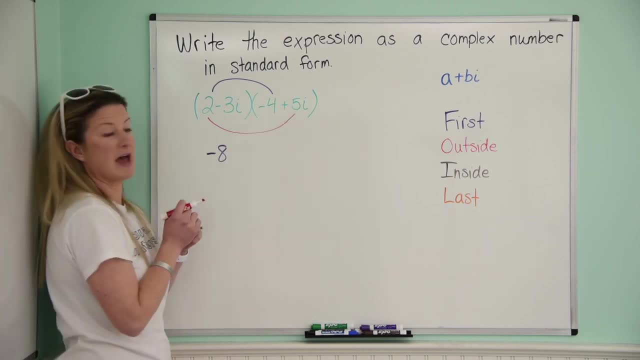 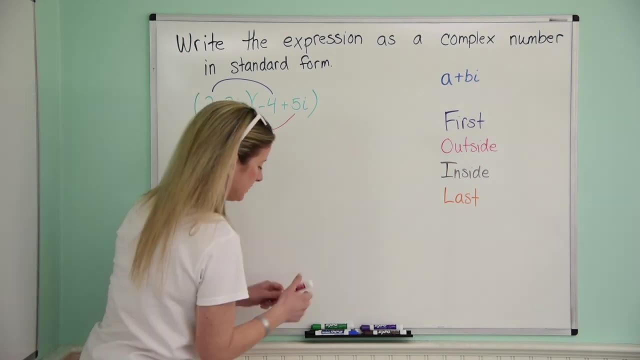 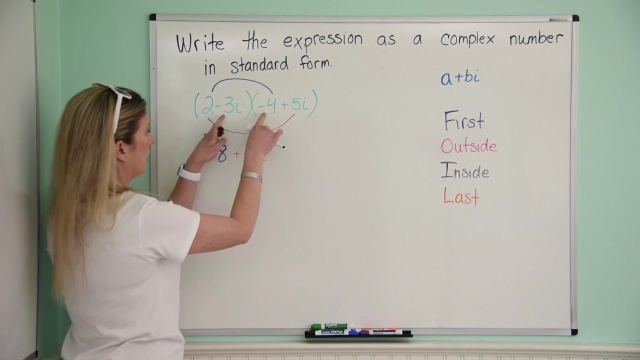 terms together: Two times five I. So two times five I is ten I. Awesome. Then inside, That was the brown one. Oops, I'll pick that up in a second. Then inside: Okay, so that's going to be our inside. 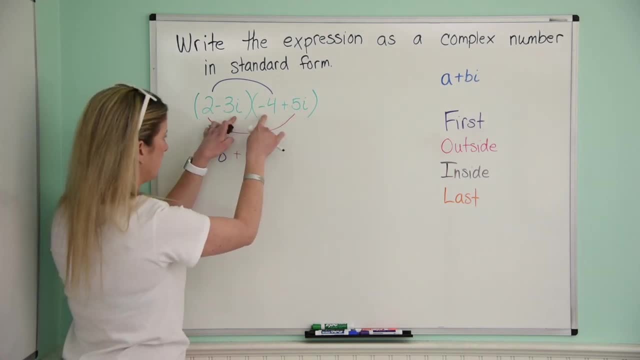 terms: right, These are first outside, inside, inside. So that's going to be our inside terms. Right, These are first outside, inside, inside. Okay, so that's going to be our first outside side terms. So that's going to be negative 3i times negative, 4.. So what's that going to be? 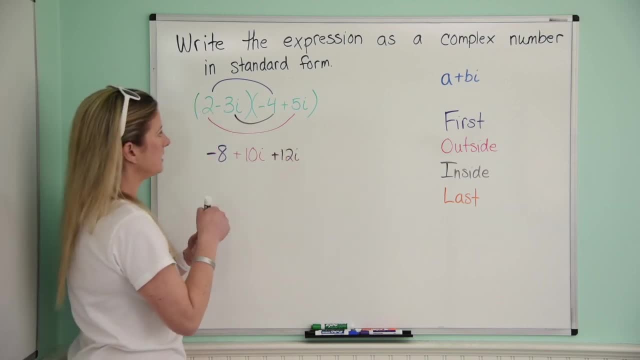 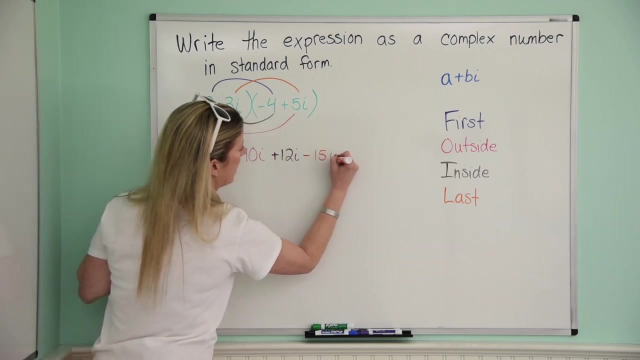 Positive 12i: Great And then last, So that these are our last terms. Okay, Our last ones. So that's negative 3i times 5i. So that's going to be what Negative 15i squared. 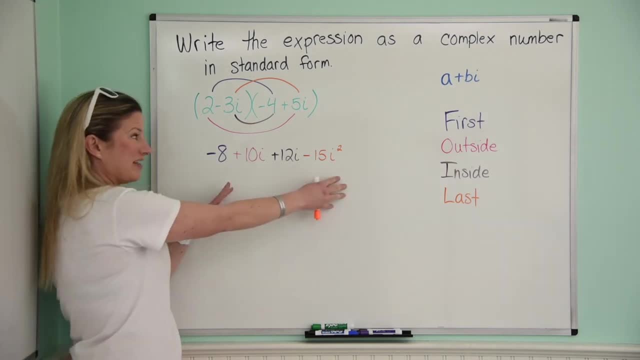 Okay, Awesome. Now we have to take all of this and get it in the form a plus bi. Okay, So we're going to combine like terms, All right. So let's see, here I've got a 10i and a 12i, So I can. 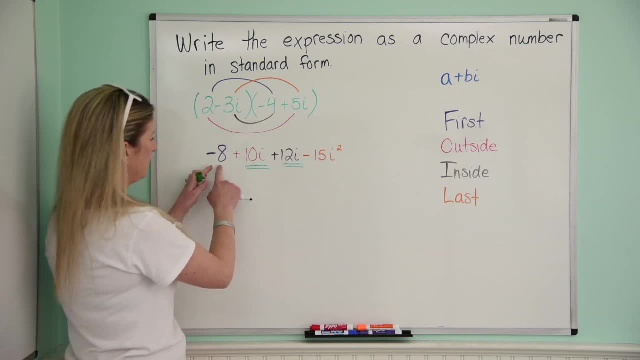 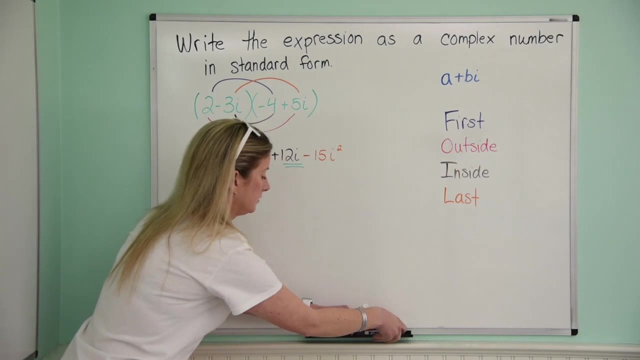 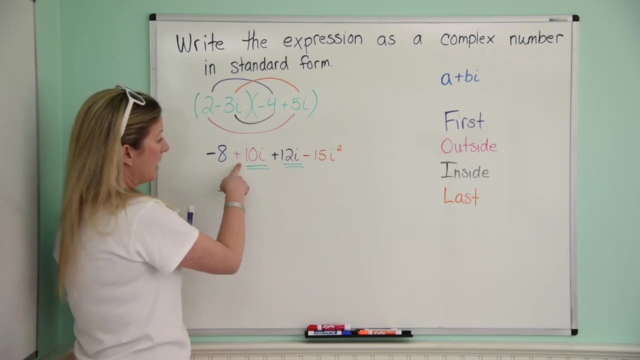 combine those, But I can't do anything with the negative 8 and the negative 15i squared yet. Okay, So let me write it as: let's do this So we'll keep the colors that we have here. Okay, Awesome. So negative 8, then positive 10i plus 12i is going to be 22i. 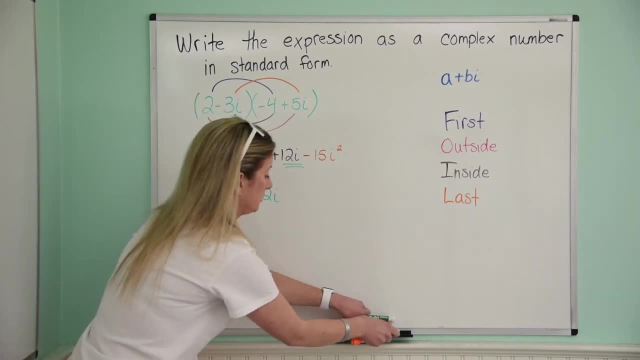 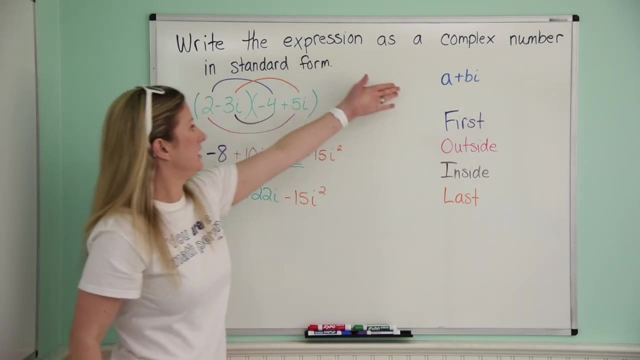 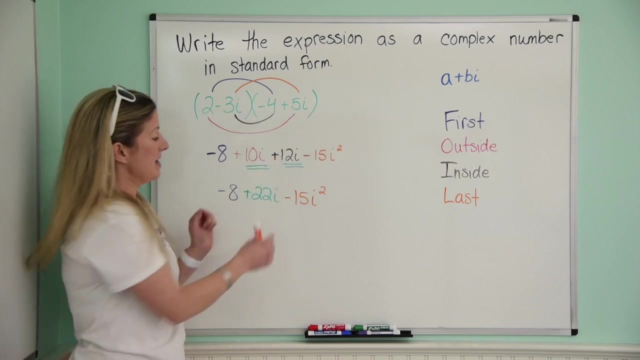 Awesome. Now I've got minus 15i squared, Perfect, Okay. So again I looked at standard form. It's a plus bi, All right. So here's the problem. There's no i squared in. that Okay, But I have an i squared here, So I got to get. 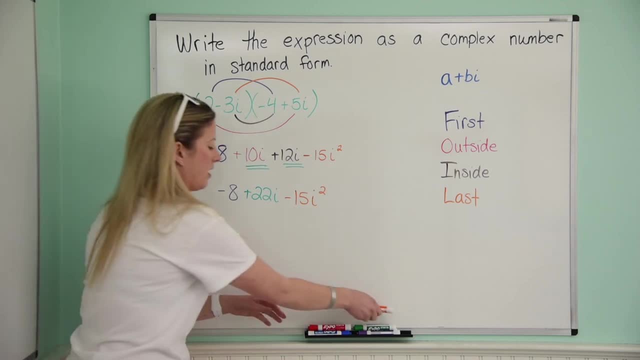 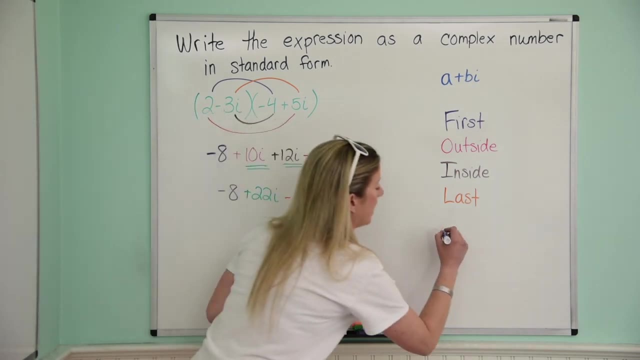 rid of it. So I have to think about how do I get rid of an i squared. Well, remember complex numbers. Okay, Remember i. All right, We know that i is the square root of negative 1.. So i squared equals negative 1.. This is so super duper important, Okay. What it means is: wherever 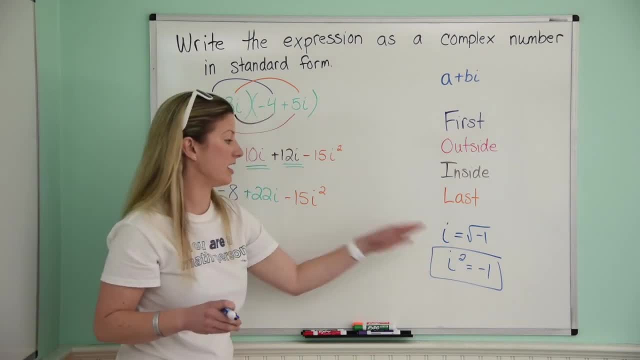 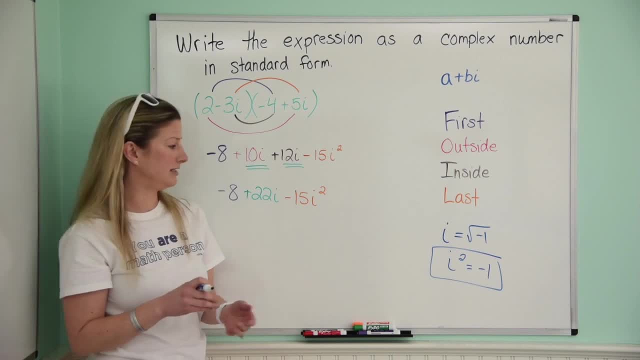 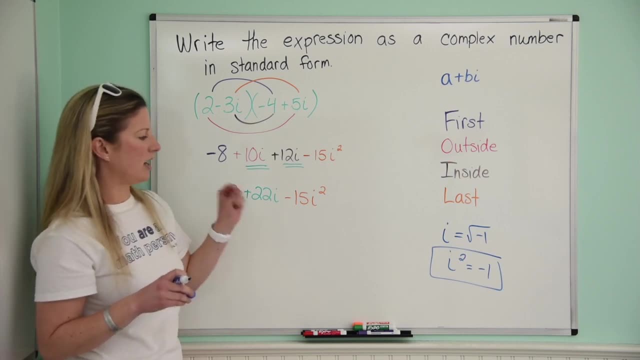 the time in the classroom and also on standardized tests like the ACT and SAT. So just always remember that If I see an i squared- and I know I'm dealing with complex numbers, you know with imaginary numbers- I know that I want to replace i squared with negative 1.. So here is 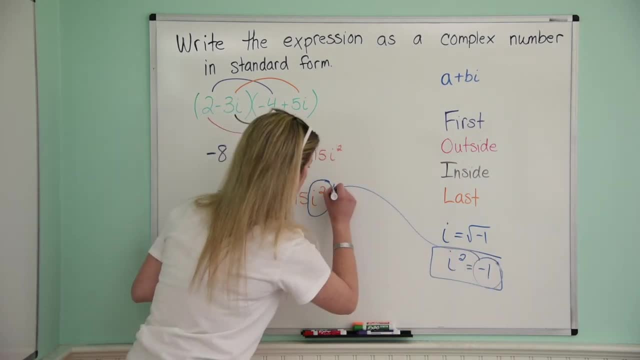 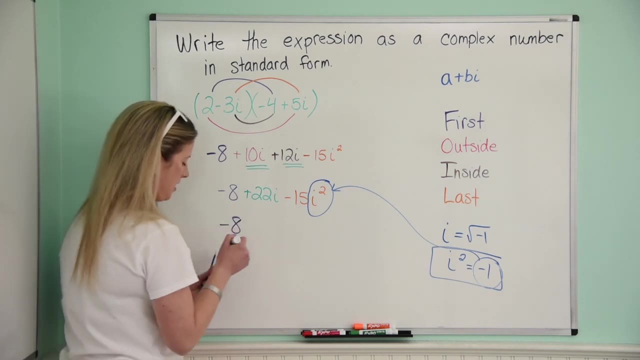 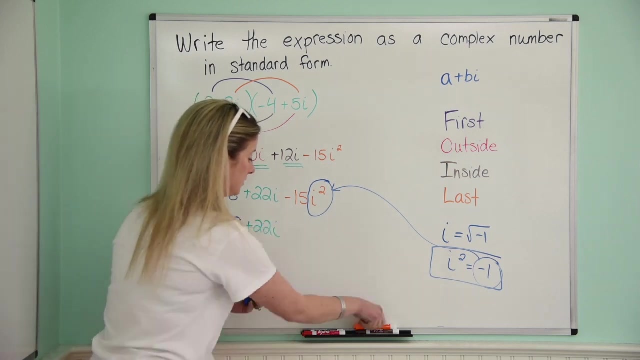 our i squared right there. So we are going to take this negative 1 and we are going to plug it in. All right, So now where's my purple? Okay, So we've got negative 8 plus 22i and then minus 15.. And then i squared is negative 1.. So we will put a negative 1 in there. 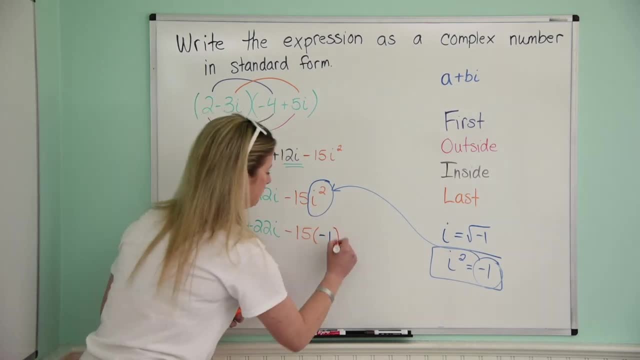 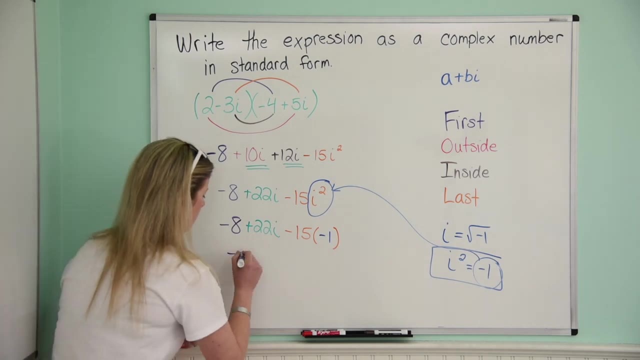 Perfect, Awesome. Okay, Now we just simplify more. So we've got still negative 8.. Negative 8 and then plus 22i And then minus. I'm going to put down the blue marker because I don't need it anymore. Okay, Minus. 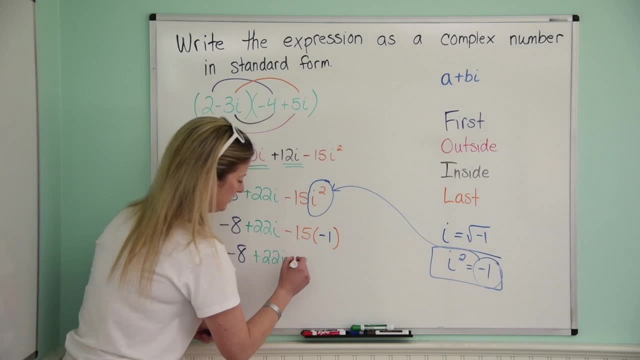 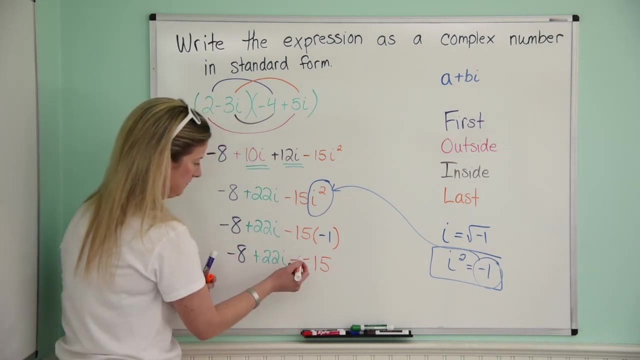 15. Okay, So minus and then 15 times negative 1 is negative 15. Perfect, So then that becomes plus, Right? Some teachers put it in as like a thing here and make it a plus, where they do plus the positive, whatever you want to do. So now look at this: We've got a negative 1 and then 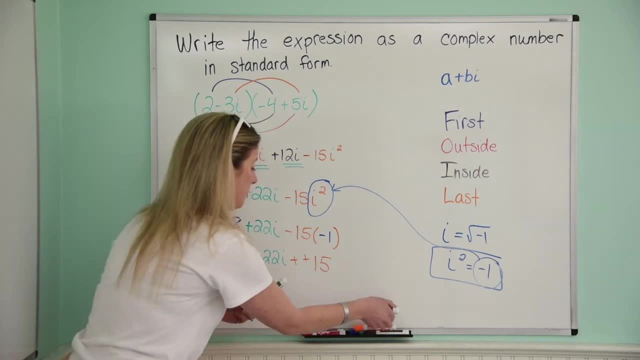 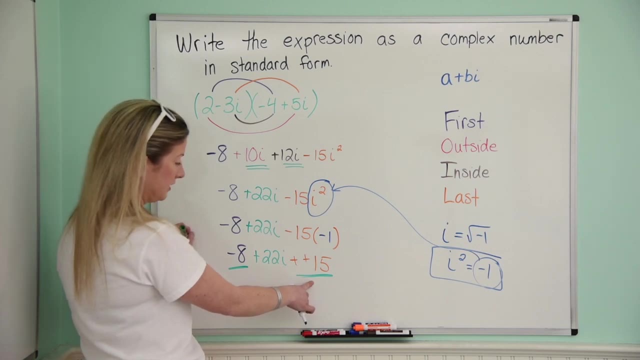 a positive 8 and a positive 15.. So we can combine like terms right there, Okay, And I'm going to use the green again, because that's what we originally started with. So negative 8 plus 15. Okay Is going.